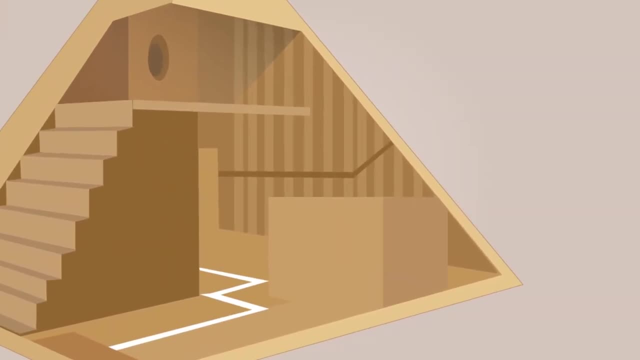 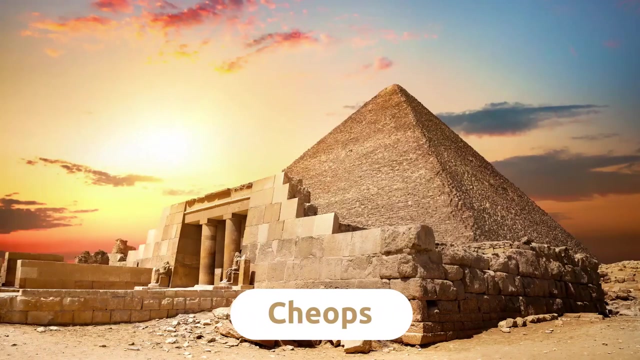 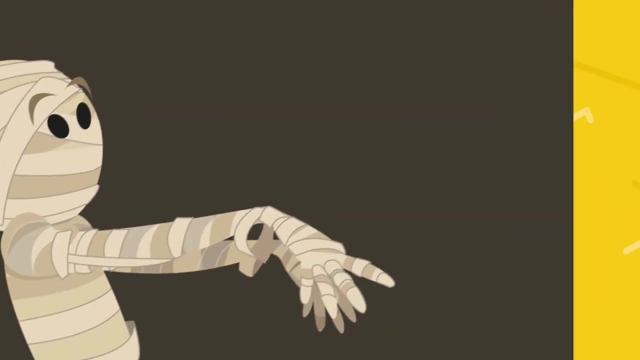 The inside of the pyramids is full of mysteries. There are tunnels, chambers and secret shafts or passageways. The most important pyramids are those of Cheops, Chephren and Menkor. What about mummies? Do you know what they were When a pharaoh or a wealthy Egyptian? 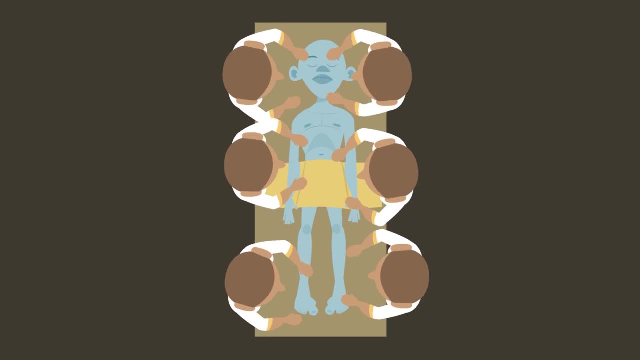 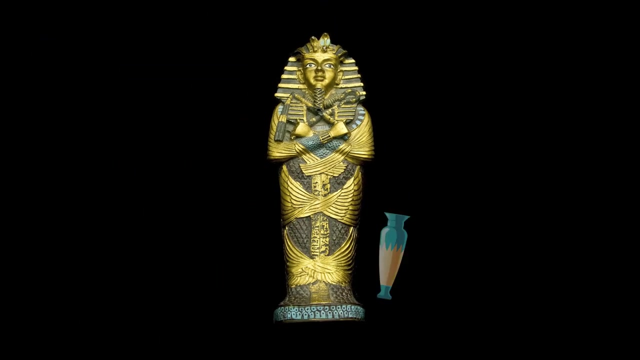 died. a body was prepared to be preserved for as long as possible. The dead body was cleaned and covered with aromatic supplements, Then it was wrapped in bandages. Later on, the body was placed in luxurious sarcophaguses. Egyptians believed in life after death. That's why, next to the dead body, they would leave. 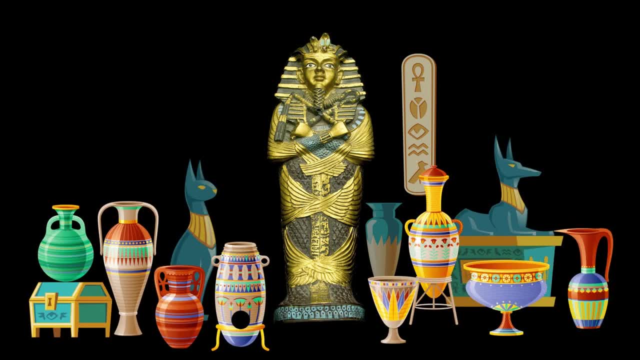 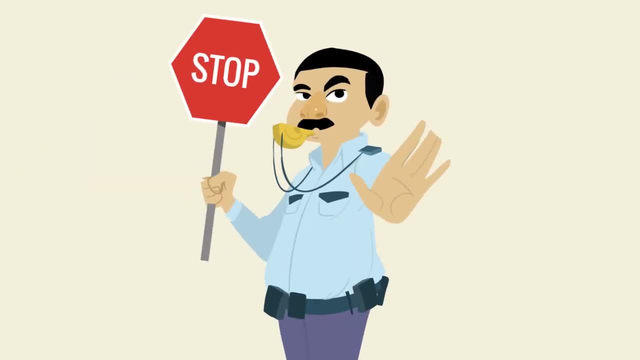 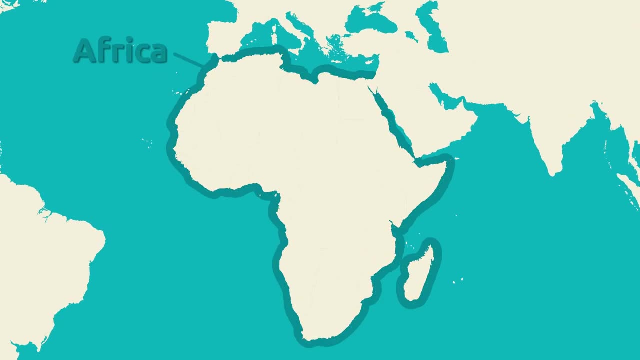 furniture, food and other objects they thought might be useful in the next life. But wait, hold on a second. When did all of that take place? The Egyptian civilization flourished in the northeast region of the African continent …in the place that is now the country of Egypt. 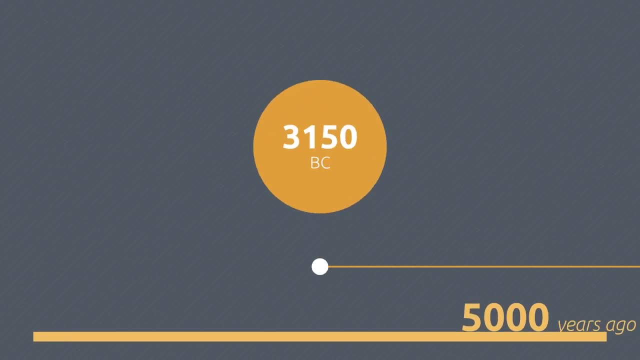 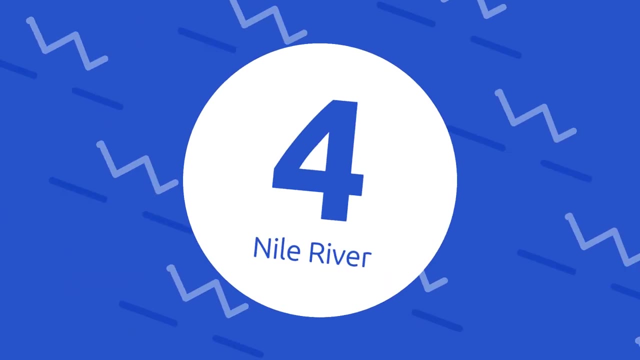 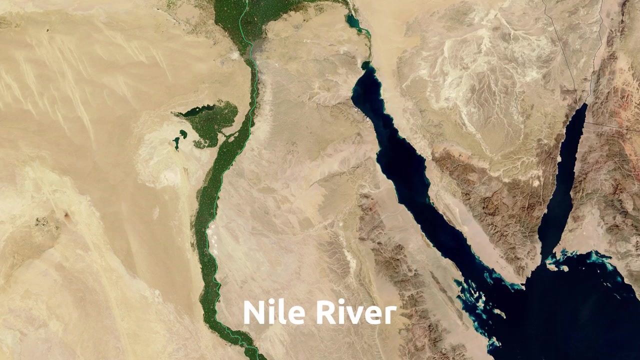 This civilization began more than five thousand years ago …and lasted about three thousand years. How impressive Climate Change. The Nile River was a key factor in the development of the Egyptian civilization. The Nile is the second largest river in the world. It is almost 7,000 kilometers long. 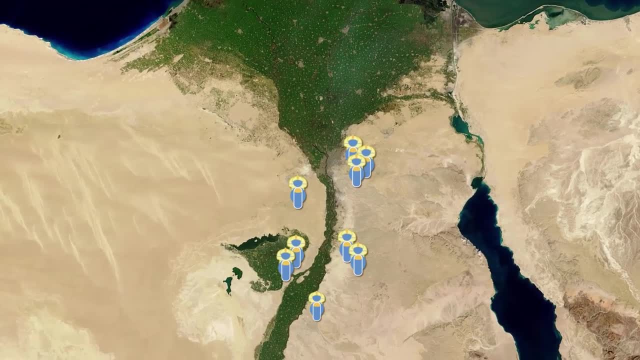 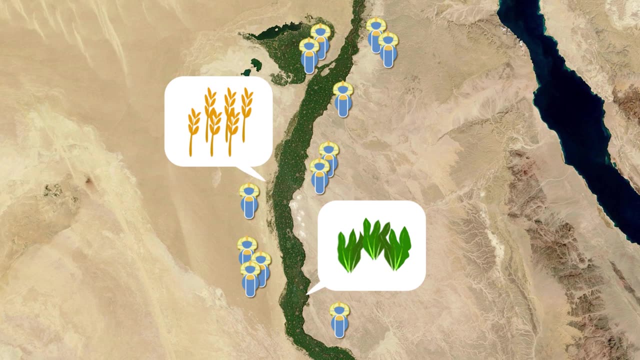 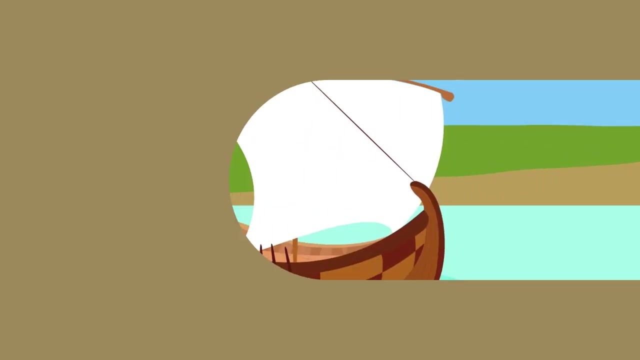 How was the developers concerned? 16,740 Emptiness flourished on its riverbanks. Egypt is mostly desert, and the few fertile lands were along the river. Oh, it wasn't just the rich harvest: People also fished in the Nile. Apart from agriculture and fishing, the Nile River was also 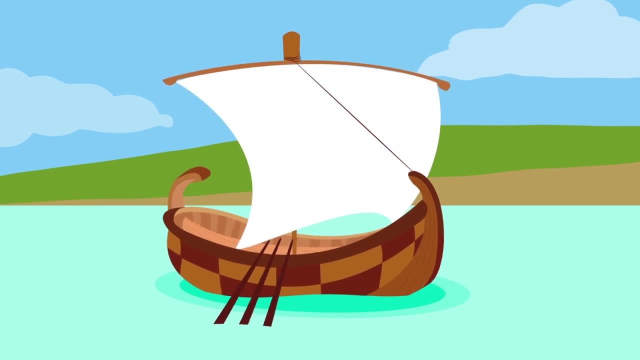 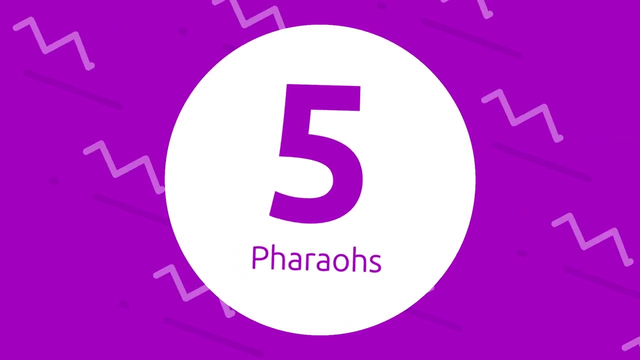 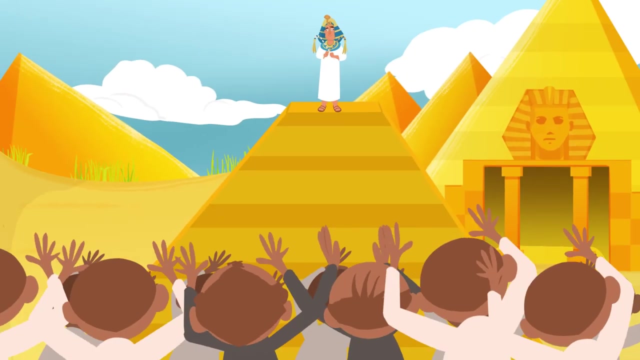 important because it was used for transportation and shipping. The ships carried people and goods throughout the empire. I'm sure you've heard about pharaohs. Do you know who they were? Pharaohs were the kings of ancient Egypt. They were thought to be gods on earth. 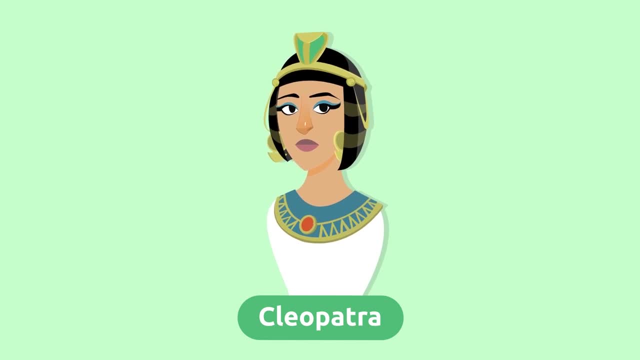 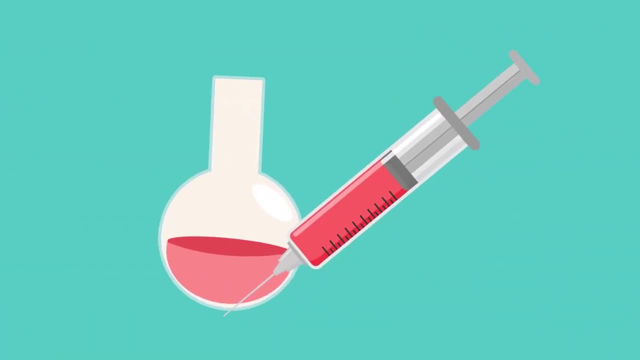 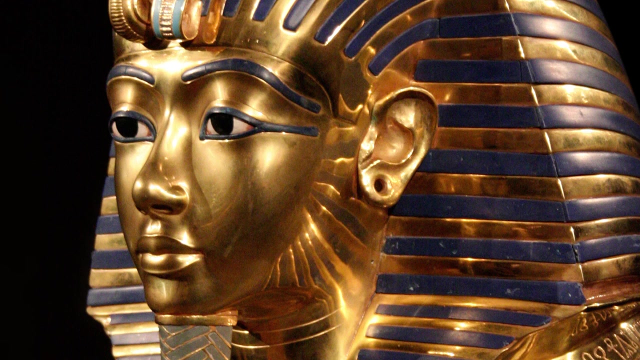 Cleopatra was one of the most famous Queens. She was also a diplomat, navy commander, linguist and wrote books on medicine. Another famous king was Tutankhamun. His tomb was discovered almost intact. Oh, I know. Did you know that King Tut became a pharaoh when he was nine years old?